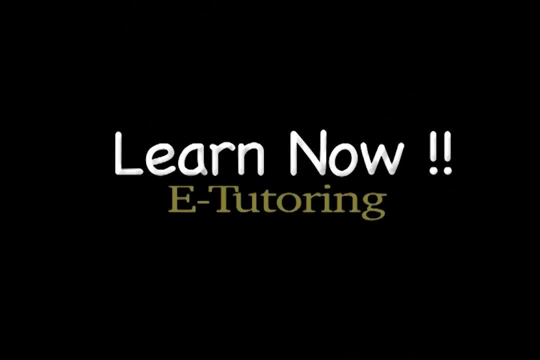 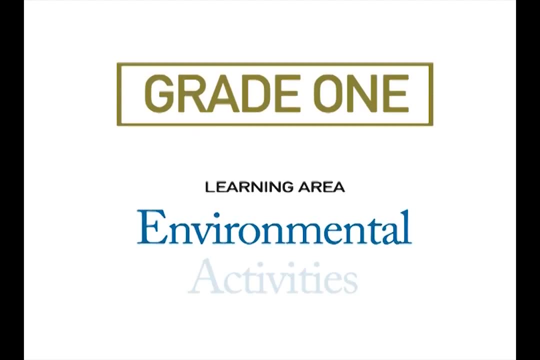 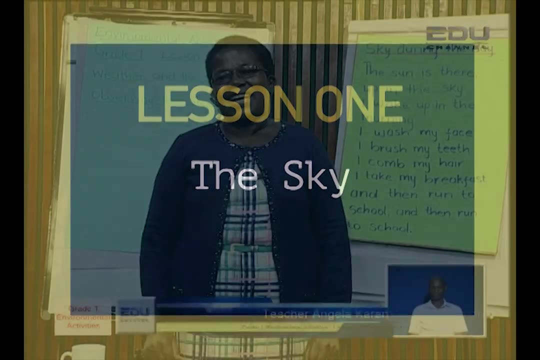 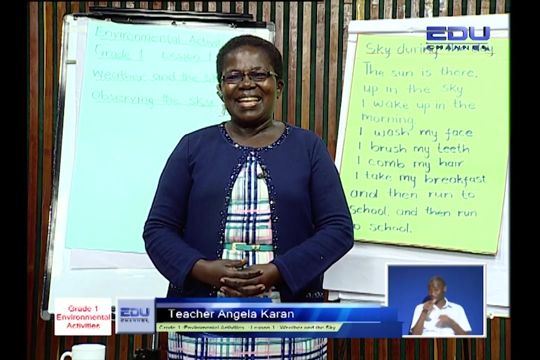 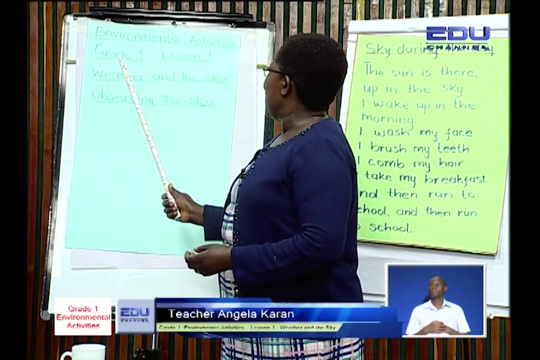 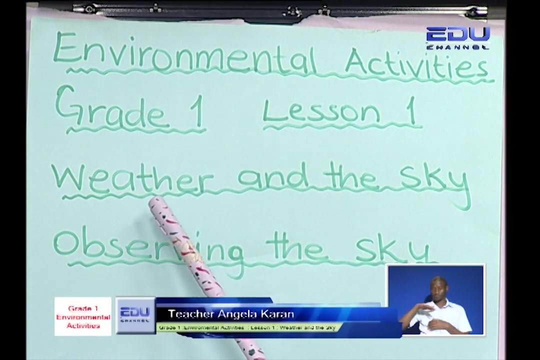 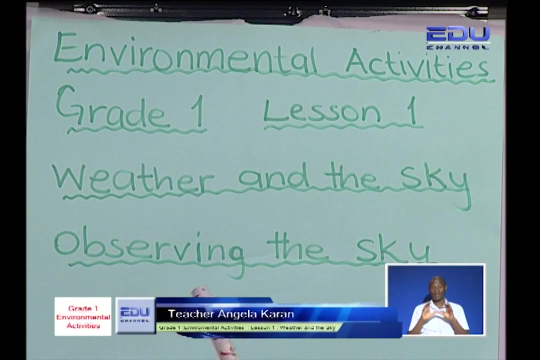 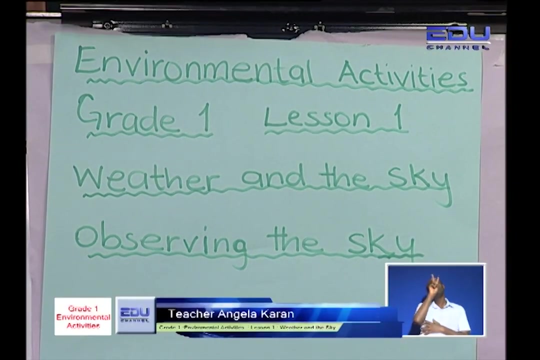 Hello Grade 1 learner. How are you today? Thank you. Today, under environmental activities, we want to look at weather and the sky, And Grade 1, we are going to observe the sky, Observing the sky. That one means that we want to look at the sky. 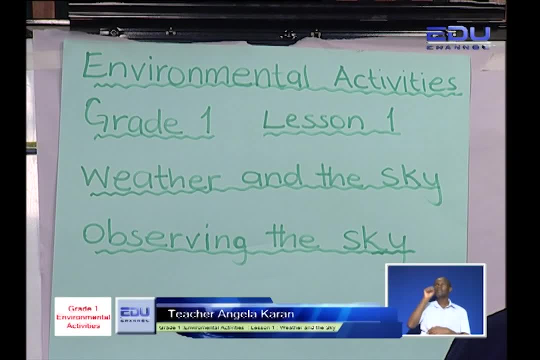 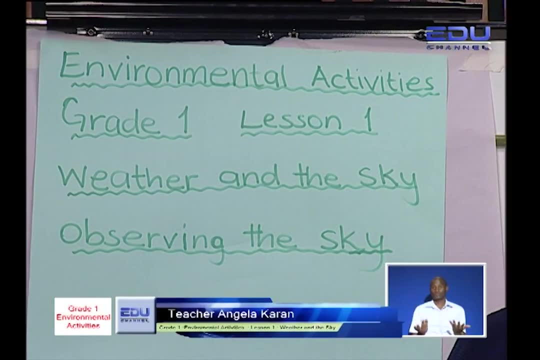 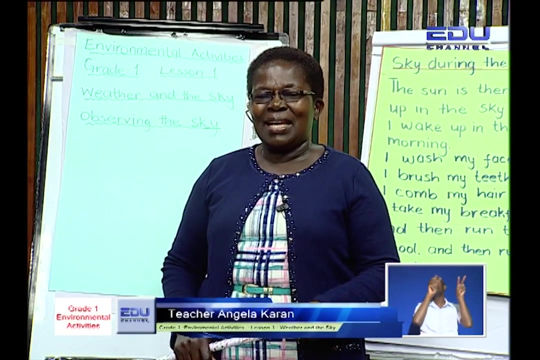 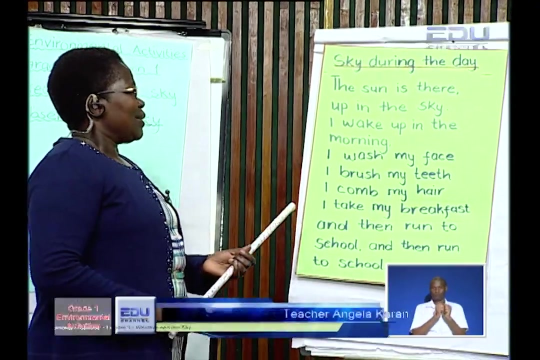 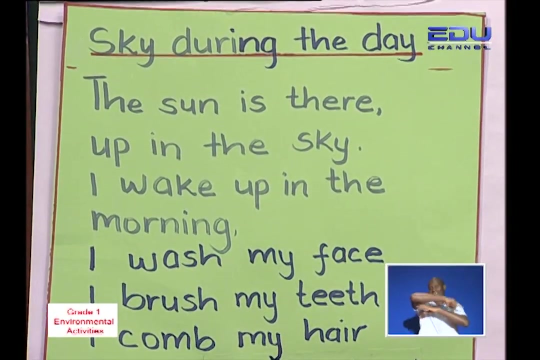 And see and mention those things that we can see in the sky. Okay, So before we start looking at the sky, I have a poem And I want us to say this poem together. The poem is about sky during the day. Say sky during the day. 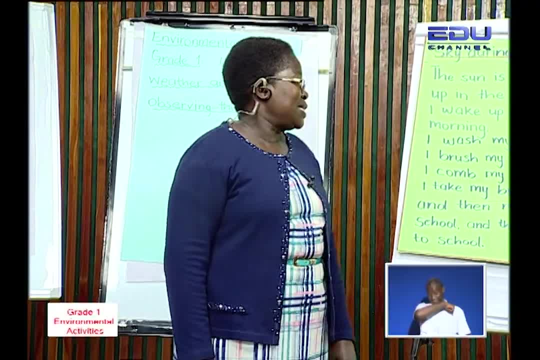 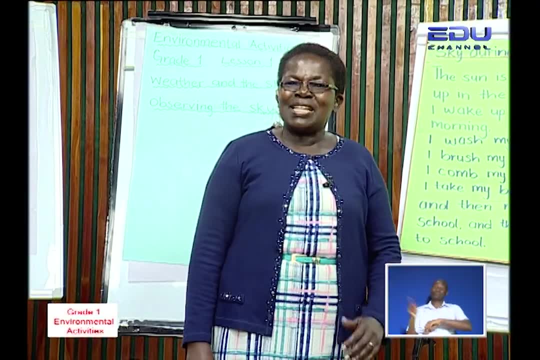 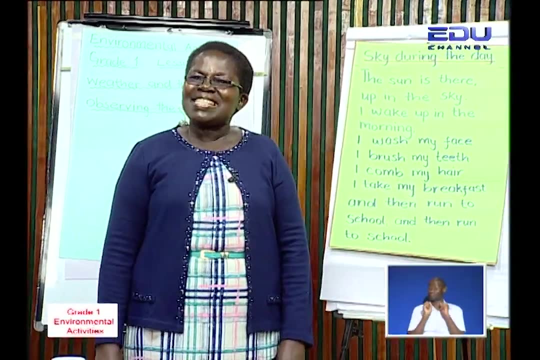 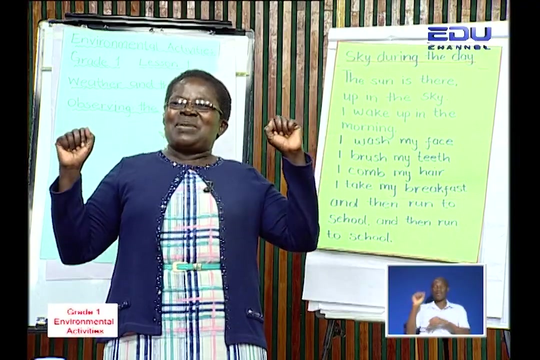 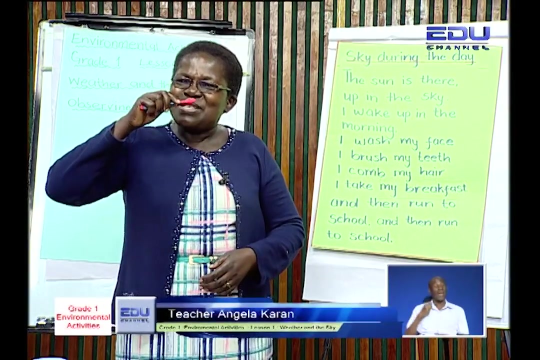 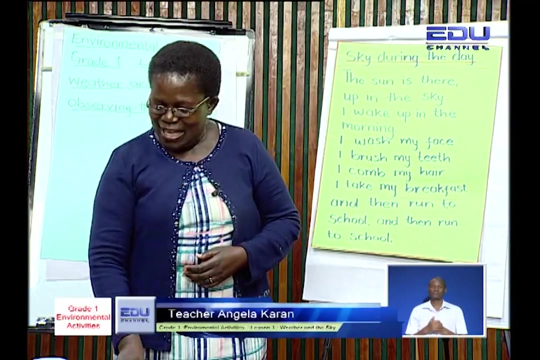 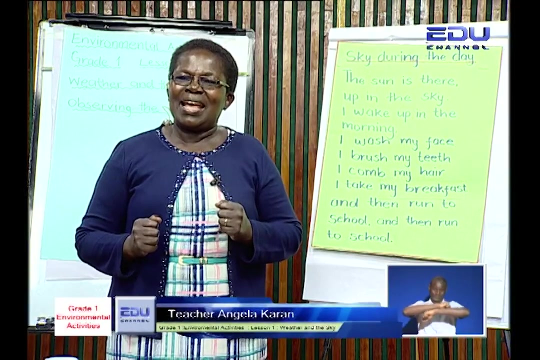 Now I want us to say the poem about the sky during the day. Listen to me as I say it first, Then we'll say it together. The sun is there up in the sky. I wake up in the morning, I wash my face, I brush my teeth, I comb my hair, I take my breakfast and then run to school, and then run to school. 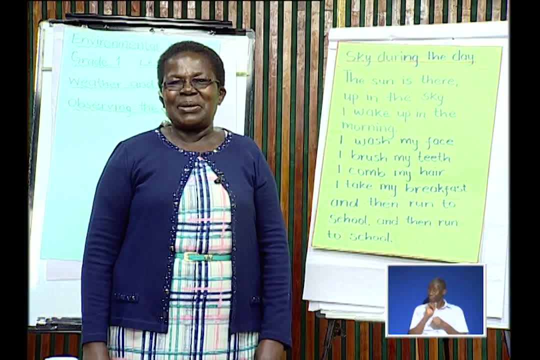 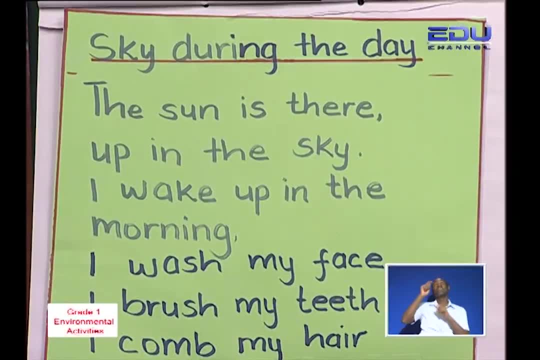 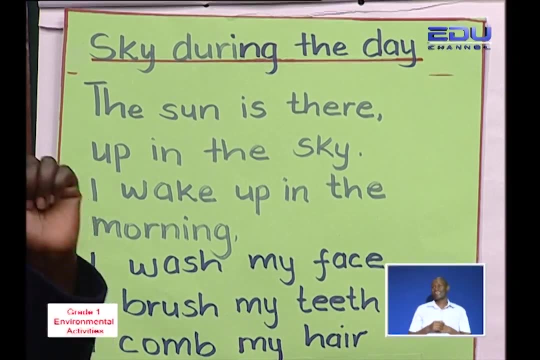 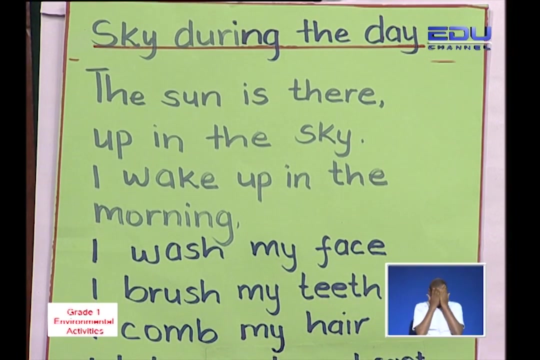 Do you do that every morning when you are going to school? Good, Now I want us to say it together: The sun is there up in the sky. I wake up in the morning, I wash my face, I brush my teeth, I comb my hair, I take my breakfast, I brush my teeth.